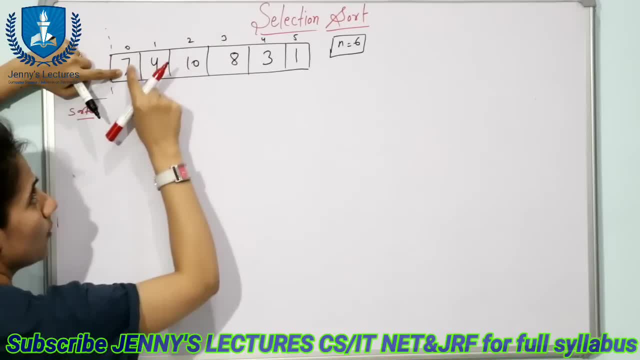 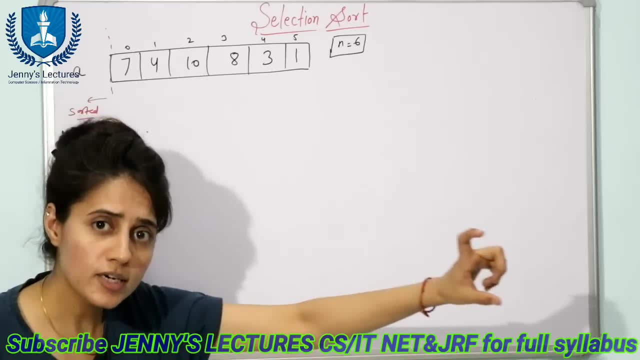 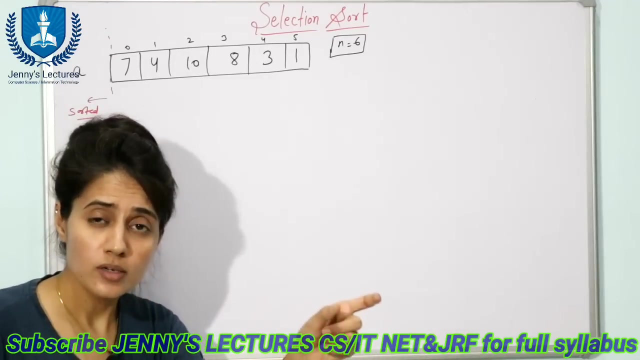 this unsorted subarray element is 7.. So this one would be swapped with this 7. One would be there and 7 would go here. Fine, So simple, funda is from the unsorted subarray. find out the minimum element and then swap with that minimum element, with the element which is: 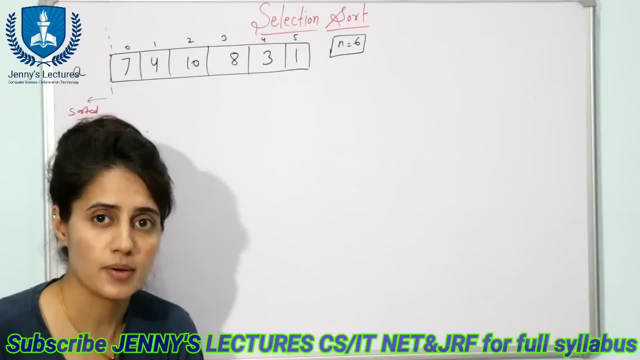 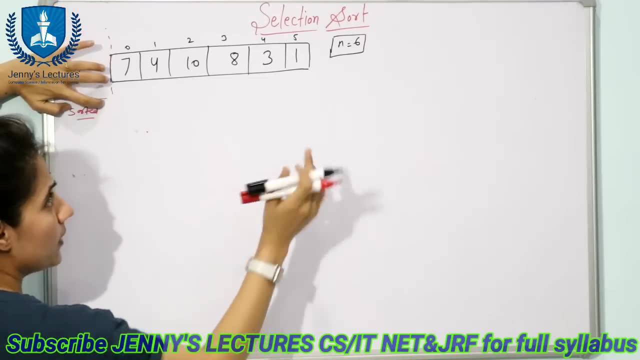 placed at the beginning, at the beginning of the unsorted subarray. See now, let us take this, this example. This is our array. Now it is starting. sorted subarray is empty, no element is there and this is unsorted subarray. This complete is unsorted subarray. Ok, So 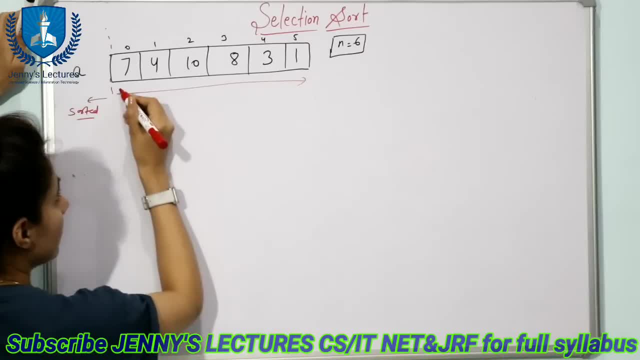 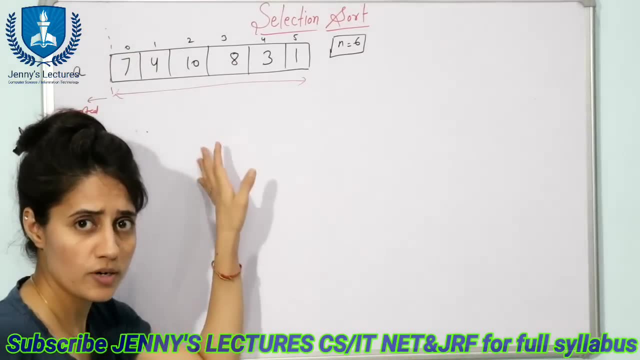 this is the unsorted subarray. This complete is unsorted subarray. Now, from this subarray, find out the minimum element. You apply the linear search. I know, I hope you know the concept, how to find out the minimum element May be the element which is at the starting. 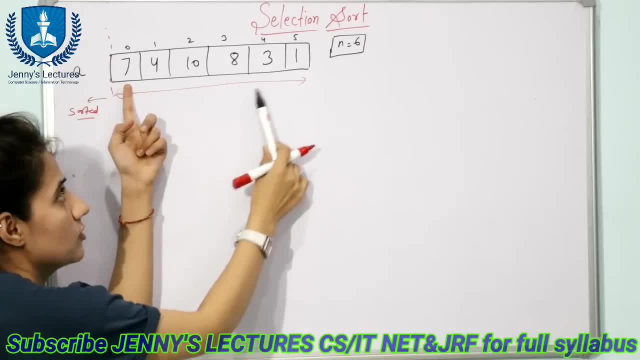 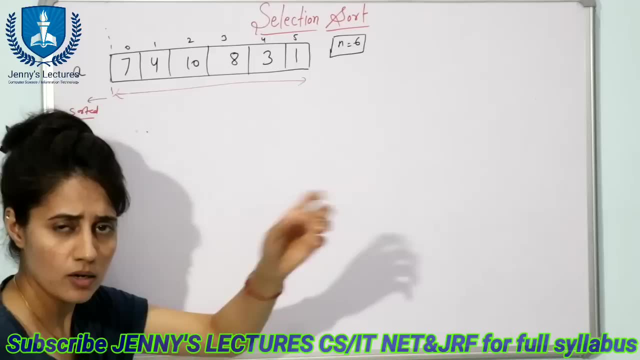 consider it as a minimum element and compare this element with all the elements, And if you find the element, one element which is less than this element, then you can consider that as minimum element. I will discuss that thing in code, in coding also. So, anyhow, by. 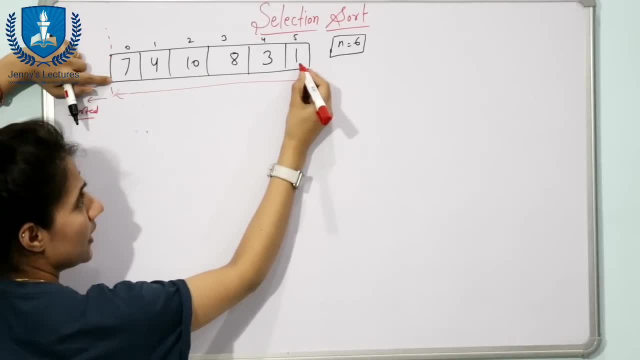 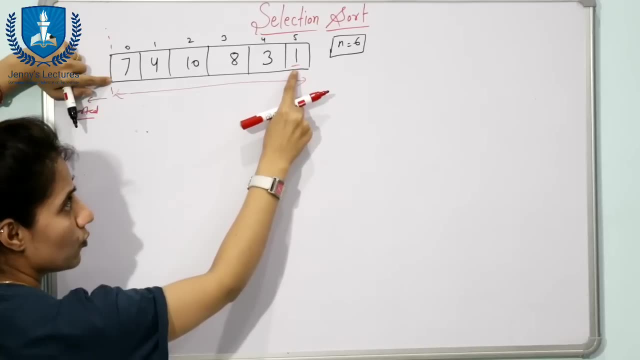 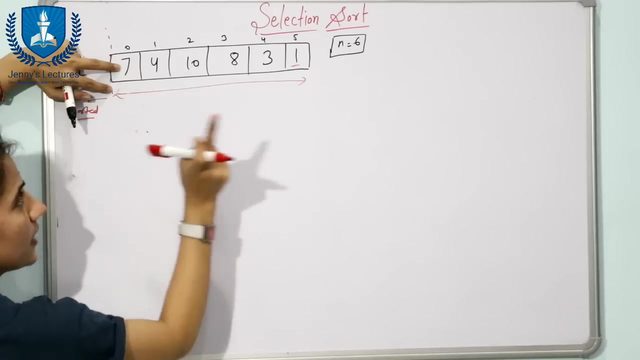 using the minimum method we have, we have found out that from this element, this a 1 is minimum element. Now next step is this: 1 would be replaced. this 1 would be swapped with the element which is at the starting of this unsorted subarray. At the starting we have element. 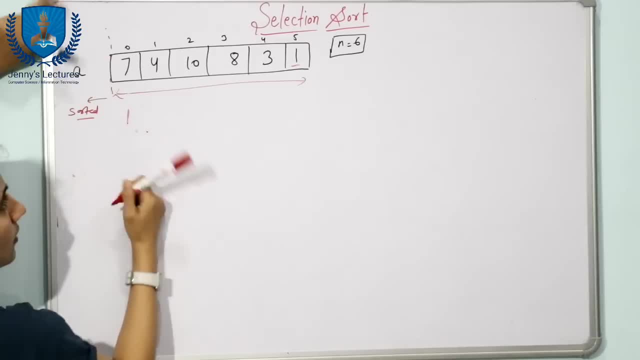 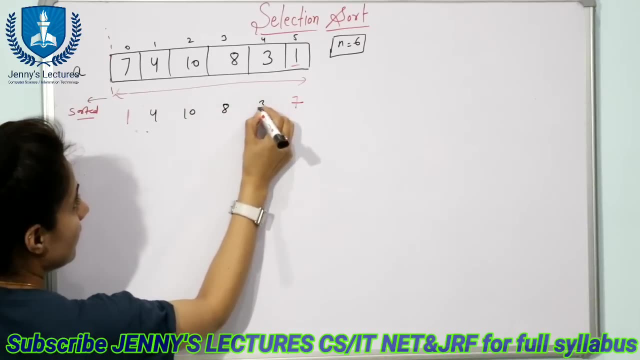 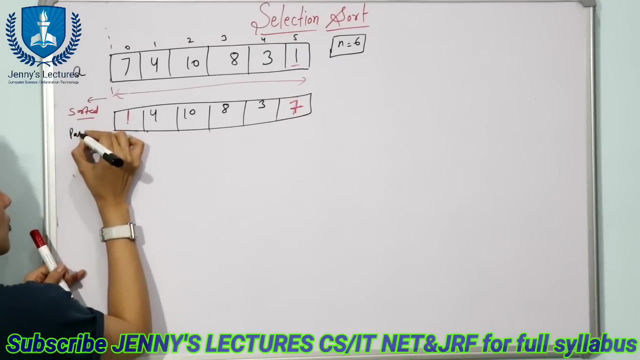 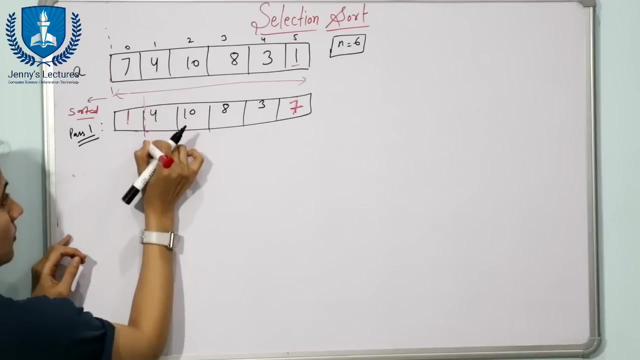 7.. So here we write what 1, and here we write what, 7.. And all the elements would be same: 4, 10, 8 and 3.. this is our array. So this is you can consider pass 1.. Now see, this is now in our sorted sub. 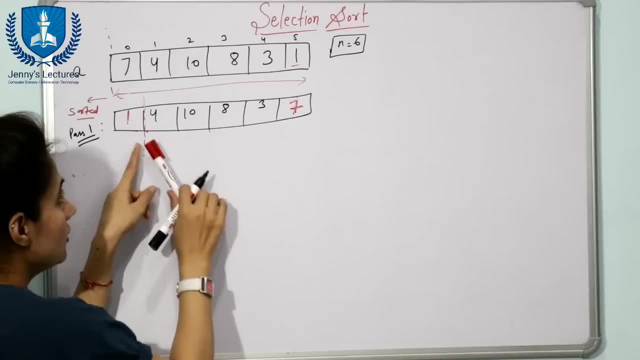 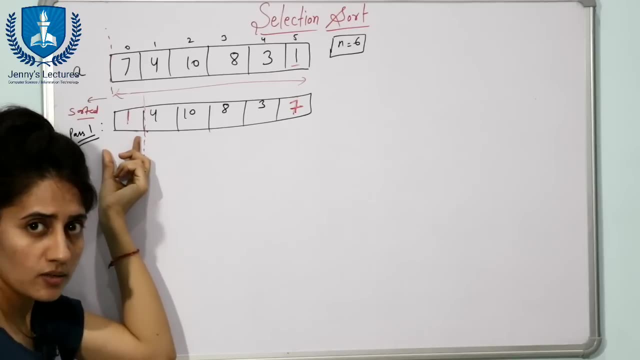 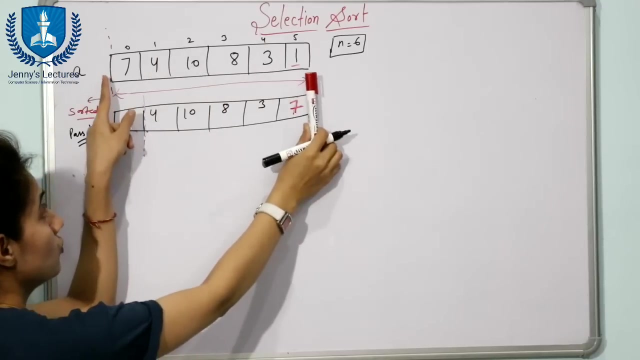 array. we have one element that is 1.. Now this is sorted sub array and this complete is unsorted sub array. Now we are going to put as it is, this sorted sub array, and we are going to deal with this unsorted sub array. Now unsorted sub array is from 1 to 5.. At starting, it was from 0 to 5.. 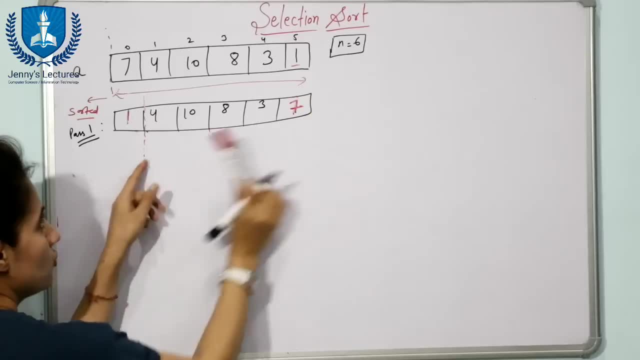 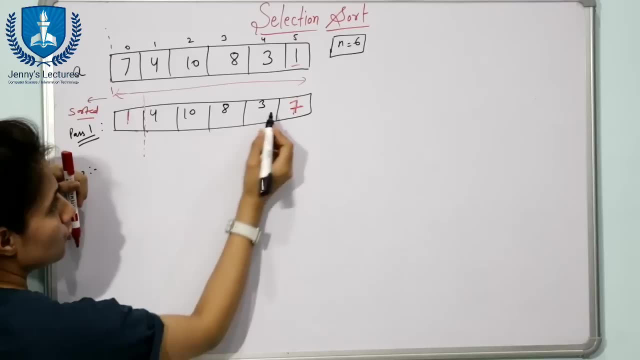 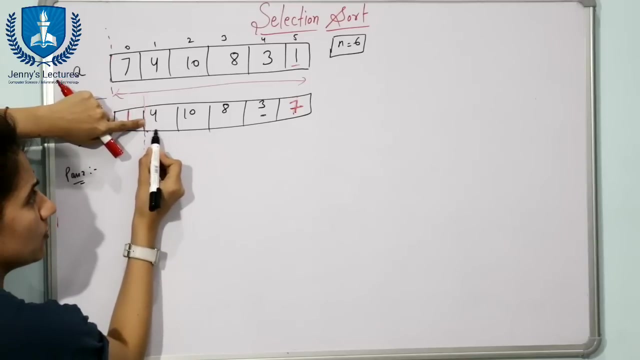 Now it is unsorted sub array. Now the next step is what in pass 2? what we will do? Same step from the unsorted sub array: find out the minimum element. Minimum element is what? This 3, and swap this 3 with the element which is at the starting, which is at the beginning of this. 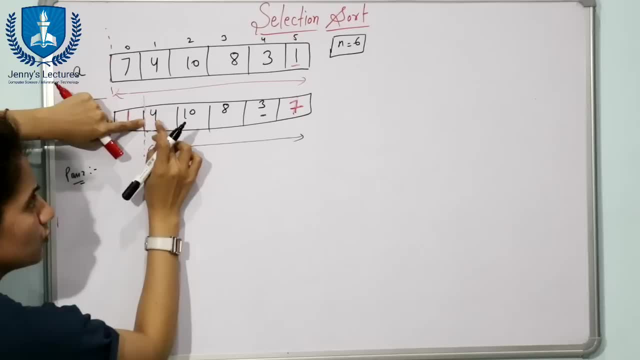 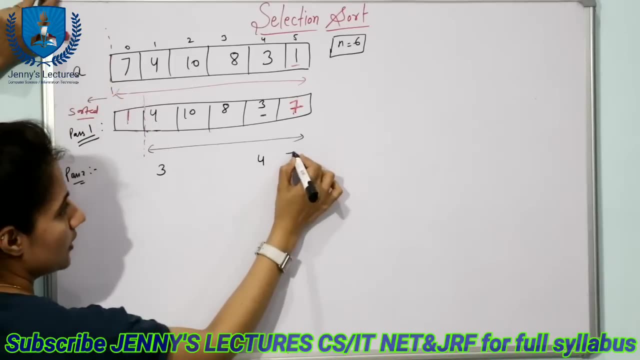 unsorted sub array. At the beginning of this unsorted sub array, the element is 4.. So what you will do: 3 would be at the place of 4 and 4 would go at the place of 3 and the remaining elements are as it. 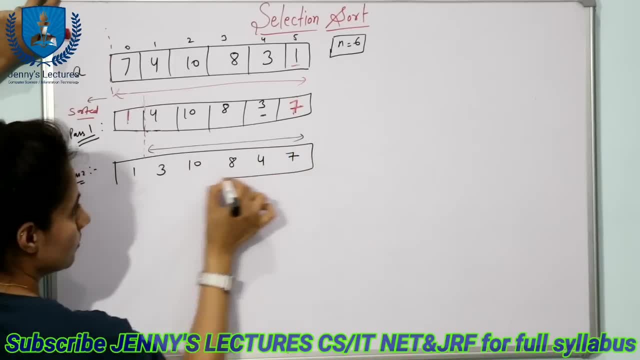 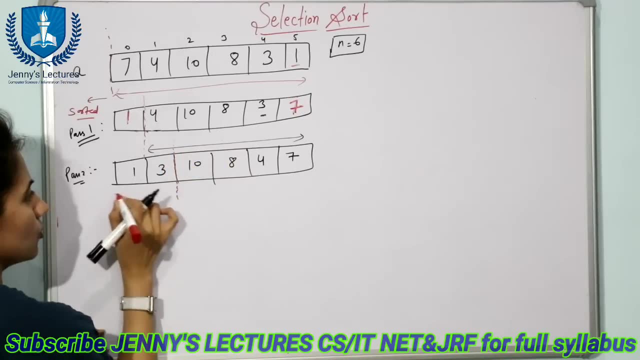 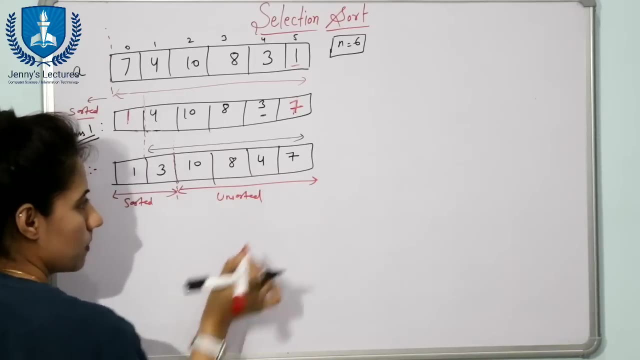 is 7,, 8,. here we have 10,, here we have 1.. Now this is the array in pass 2.. So now this is now sorted sub array and this is now unsorted sub array. Fine, Now you keep it sorted sub array as. 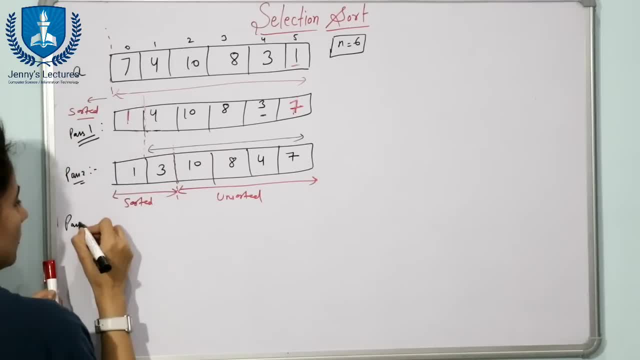 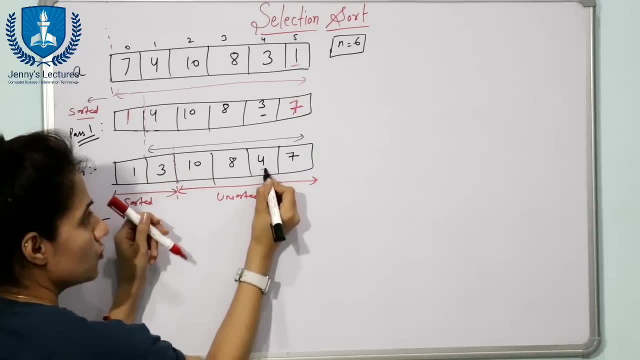 it is, and you deal with this unsorted sub array In pass 3, what you will do From this unsorted sub array? find out the minimum element- Minimum element is what This? 4- and place this minimum element or swap this minimum element with this. 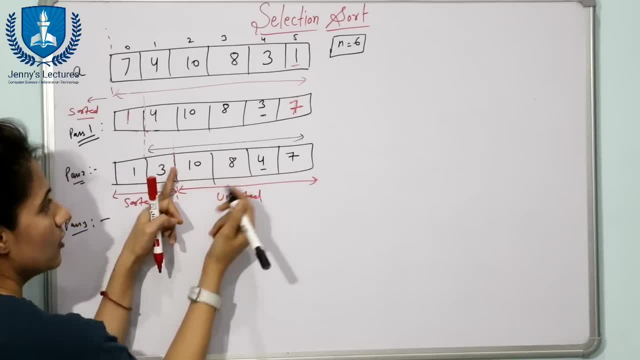 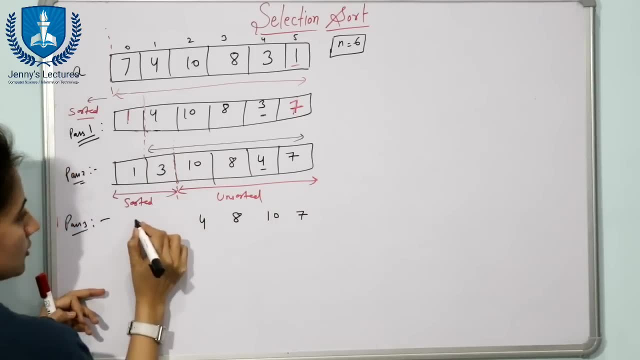 10, because at beginning of this unsorted sub array the element is 10.. So what you will do: 4 will go here and 10 will go at the place of 4.. All the elements would be as it is: 1 and 3.. Now 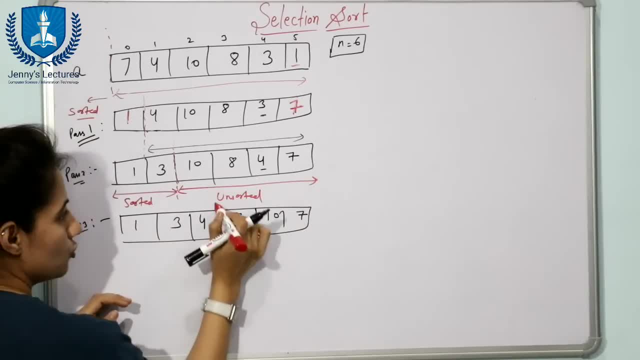 this is the array Now. you will keep it sorted sub array in point 5.. So at the anni 1 we took the starting point 이렇게: the partition pick out 2 at point 1 and we check it again. 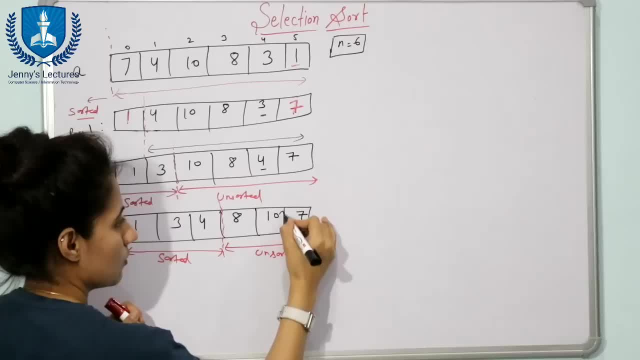 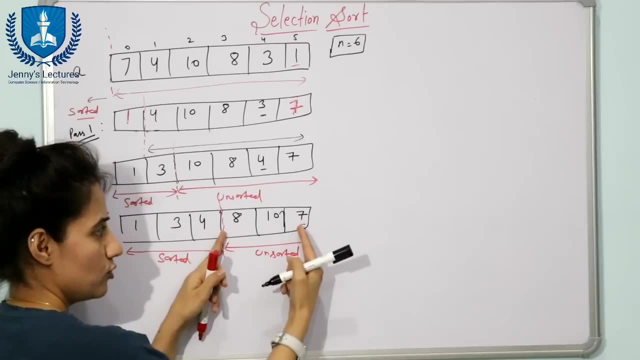 What will you do? We take the starting point and write M Where M of us should go. we will put up N spoke into M of state. We will repeat anytime we change it here, As we can see theugar strength Now, when you remove the data, this is just as it has been So. 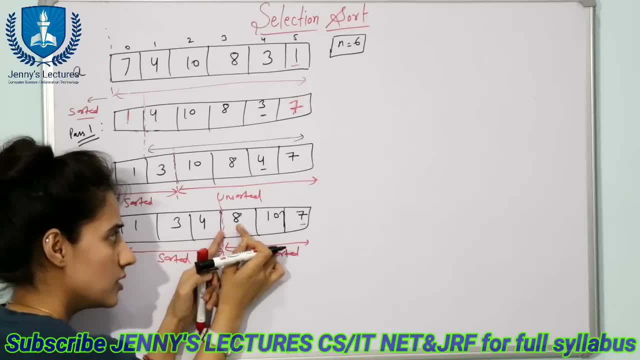 first of all, we were saying that the value of question is equal to min 1. Little bit of margin does not matter. the morally important information is what makes all the data common. When we come toила, we take h it its location. so the value is like this: If the value of 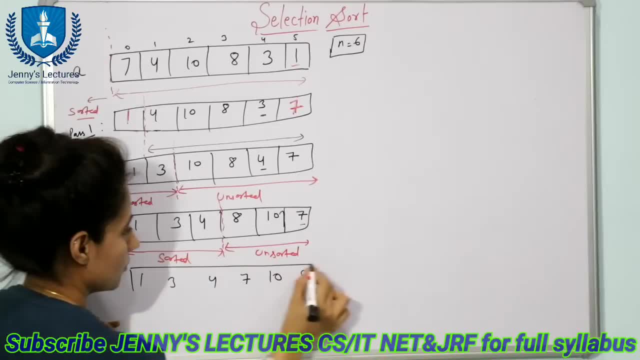 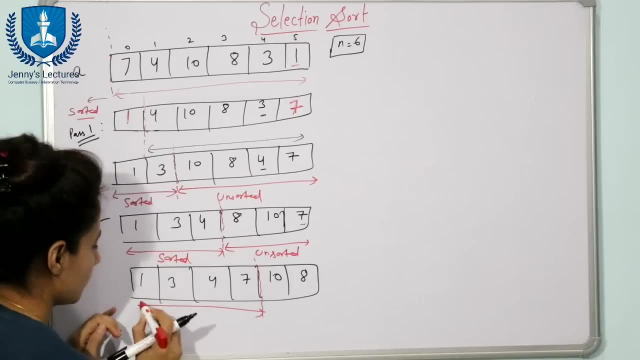 нимt here and the bottleneck here and remaining element will be, as it is, 1 total It isbal hometown is minus theta right, minus theta square, Tong i Leon minus side health. minimum element: it is 1,, 3 and 4.. Now our sorted subarray is this much and this remaining two elements. 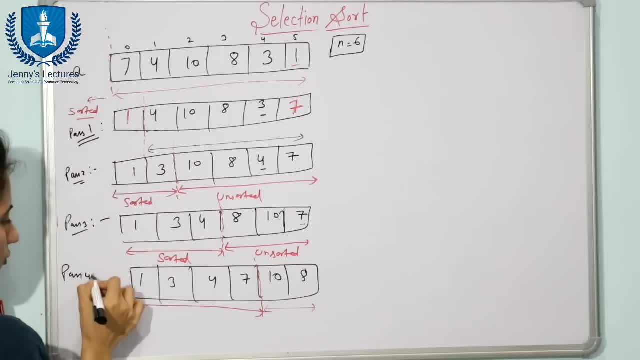 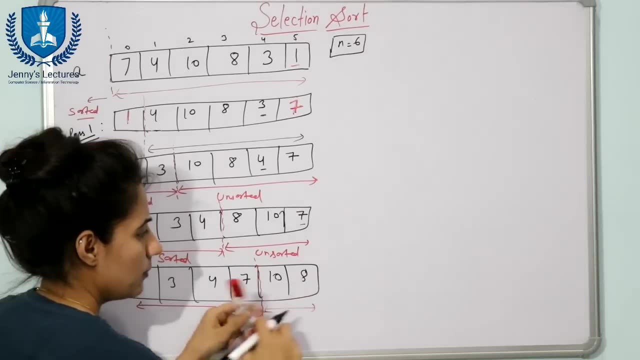 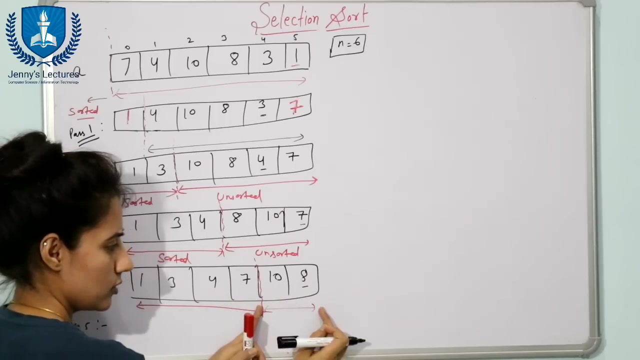 are in unsorted subarray, and this is pass 4, and in pass 5, what you will do from the unsorted subarray. find out the minimum element- minimum element is 8- and swap this minimum element with the element which is in the starting of this unsorted subarray, At starting of. 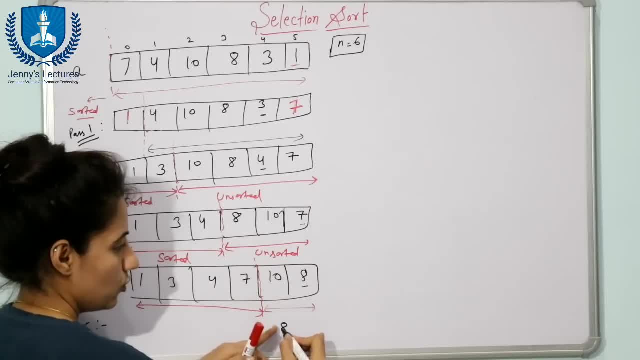 this unsorted subarray. we have 10, so we will swap out this one: 8 would go here and 10 would go at the place of 8, remaining element would be 7,, 4,, 3 and 1.. 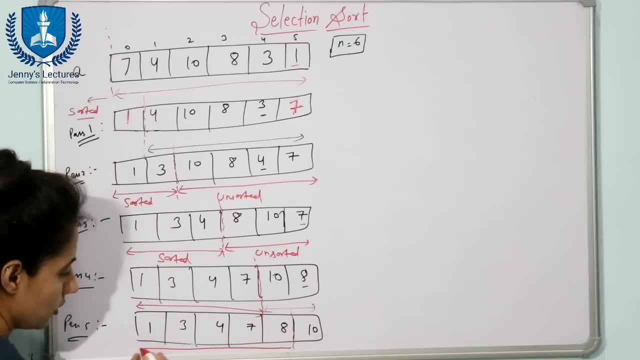 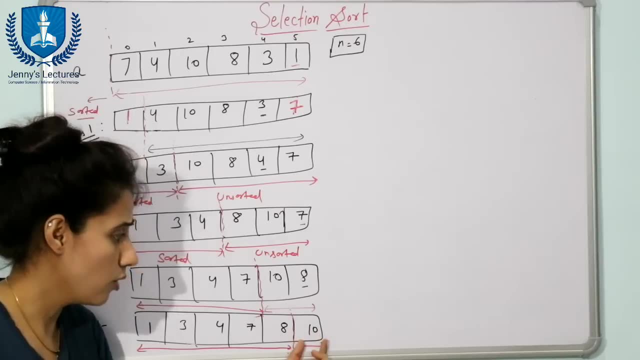 Now see this: this much is sorted subarray, and in unsorted subarray we have only one element. fine, So no need to sort this one, because if one element is there, then obviously that is always sorted. So you can say that if 6 elements are there. 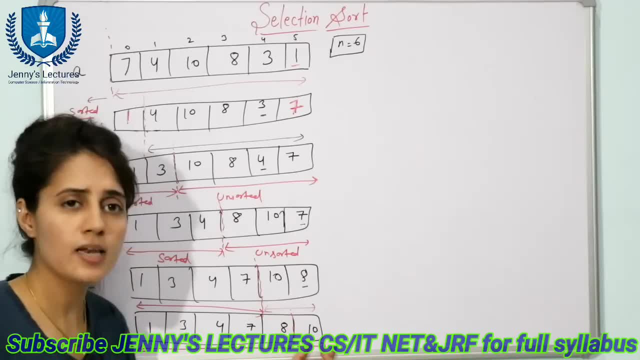 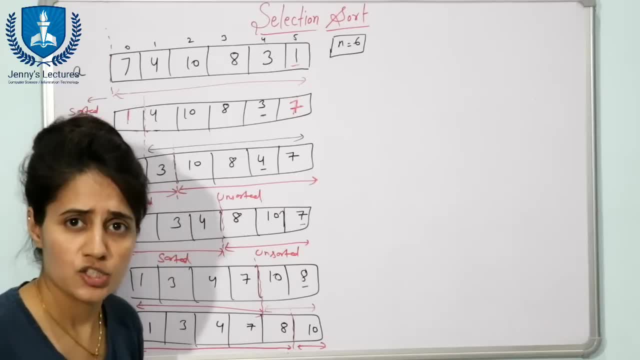 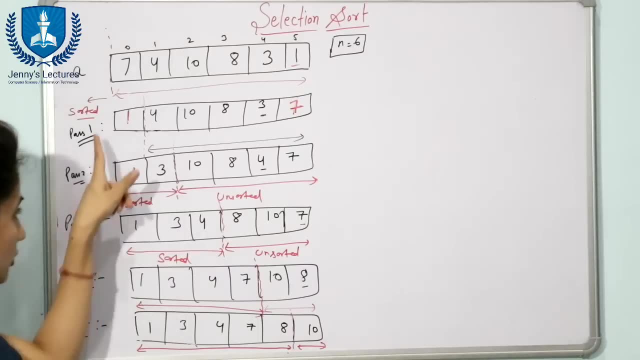 no need to sort that element. So this is the funda of selection sort. okay, now how to write down this into code here. two loops would be there. one is for this passes. five passes are there means n minus one, so outer loop would be for these. 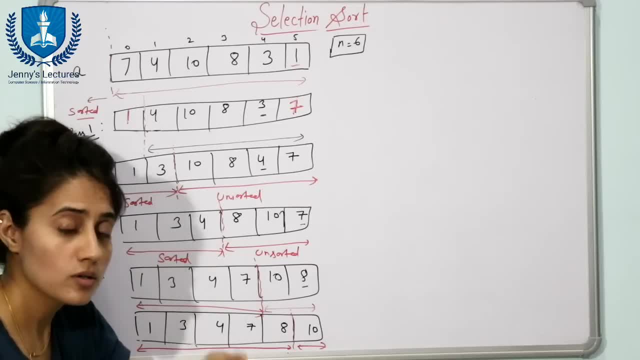 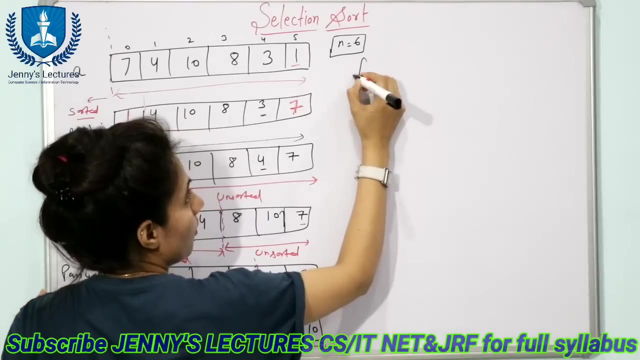 passes. and second element is what? sorry, second loop is for what? to find out the minimum element from the unsorted array and for the swapping, or you can say, to find out the minimum element from that array. okay, see, now after loop would be from: i is equal to zero, to be less than n minus one. 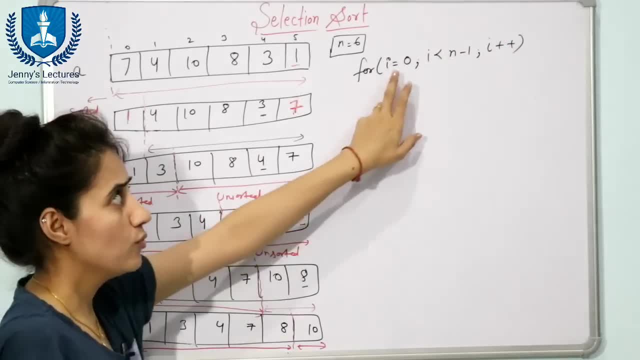 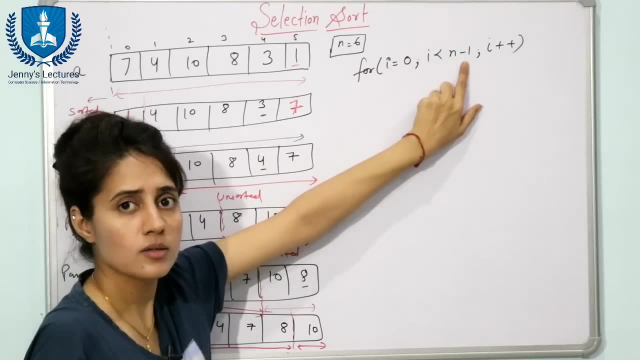 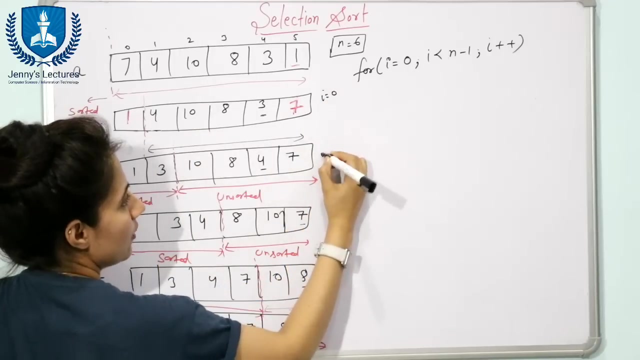 and i plus plus. so this loop is for this passes. passes is five. so we will start from zero to less than n minus one. n is six, six minus one is five. okay, so i value would be from see in pass one: i value is zero here, i value is one here. i value is two. here i value is three and i. 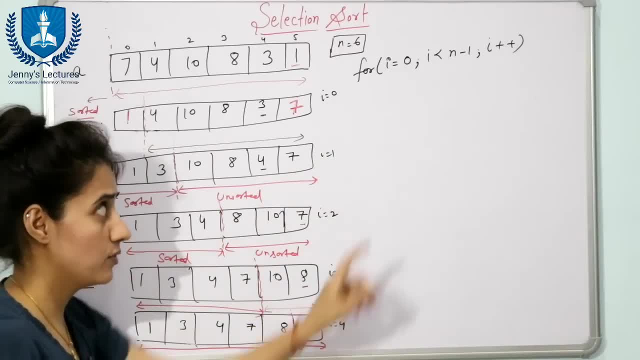 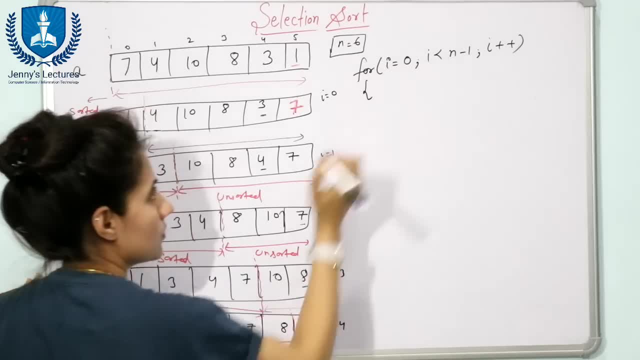 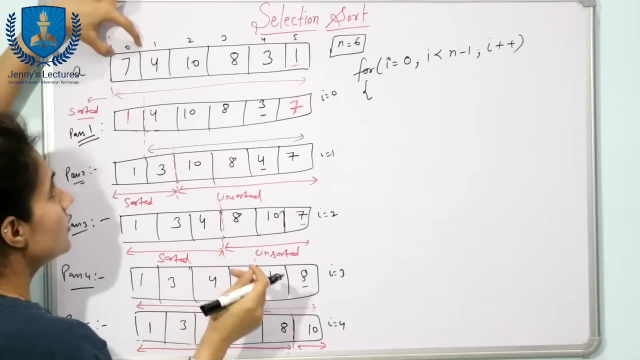 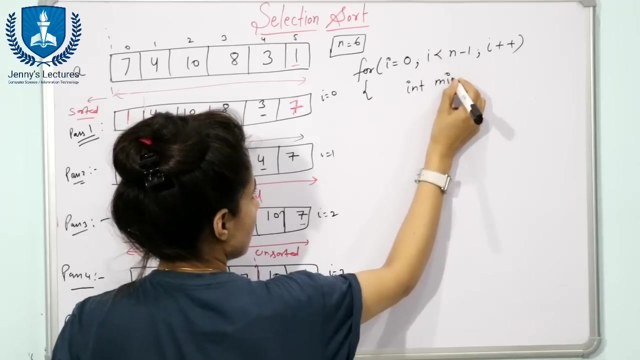 i have written less than n minus one. fine, now see next what you will do: how to find out a minimum element. first thing is, just consider the first element is the minimum element. okay, now see what we will. take one another variable min. we will initialize this min with the value that is. 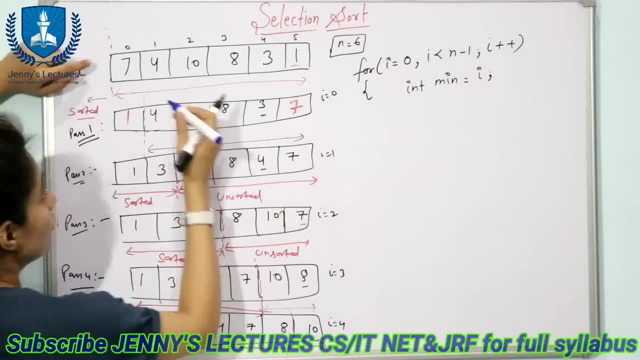 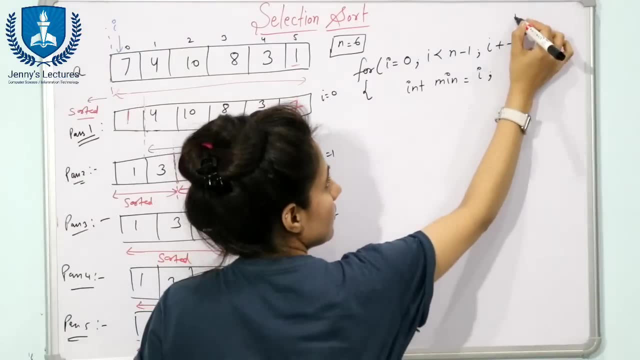 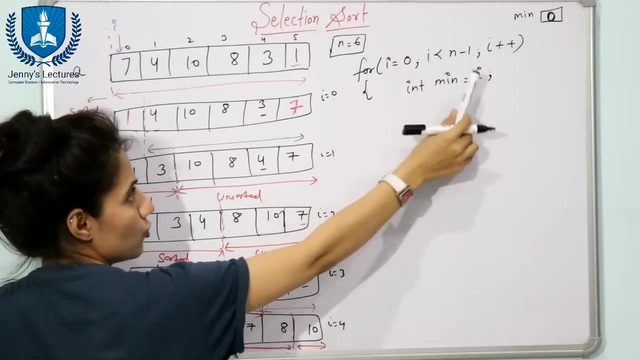 i value. okay, so now see at start when i value is zero. i is here and min. min is a variable and min is the value. of min is also zero because i is zero. so here we have zero. now what you will do now: you will compare this. 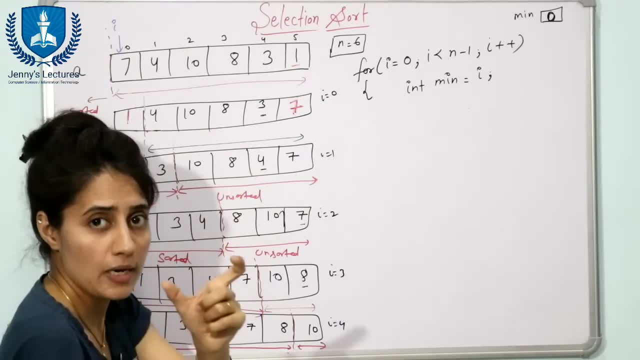 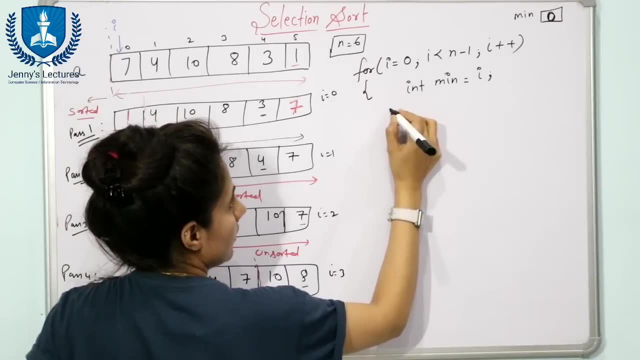 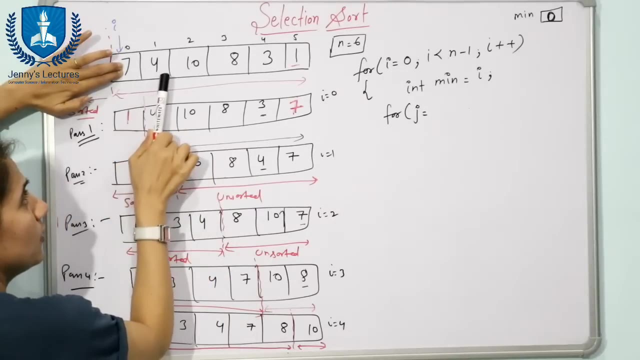 element with these elements to find out the minimum element. i hope you know the concept: how to find out a minimum element, how to search, how to do linear search. see now, for example, we are going to start another loop and we are going to compare this element with this one. so 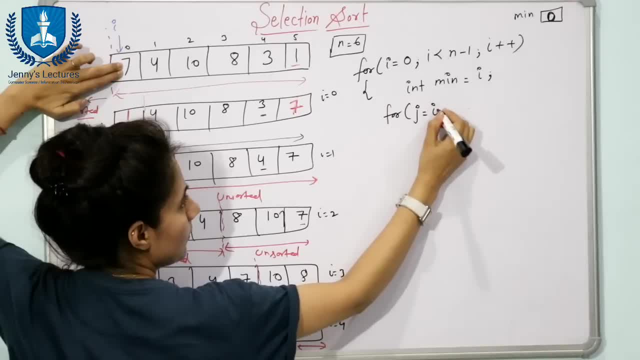 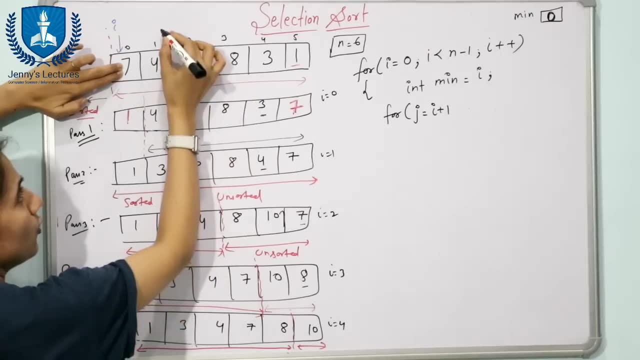 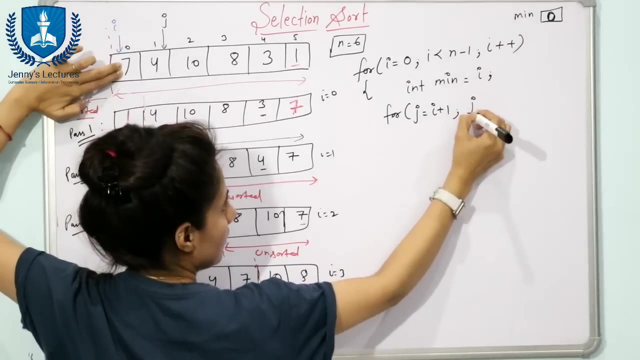 we are going to start from here. so j would be i plus one. we are going to compare this element with this element, so this element is at index i. so we are going to start from here. so j is starting from here. only j is equal to i plus one, and j would go till what less than n. 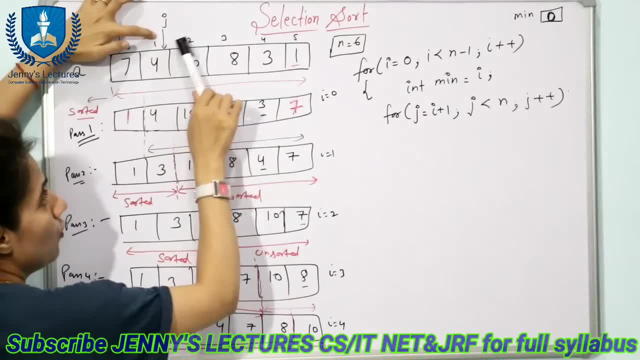 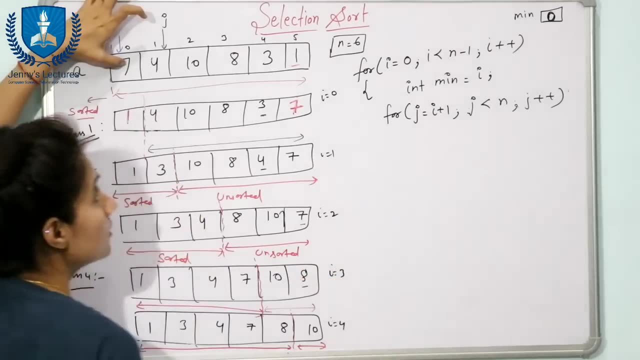 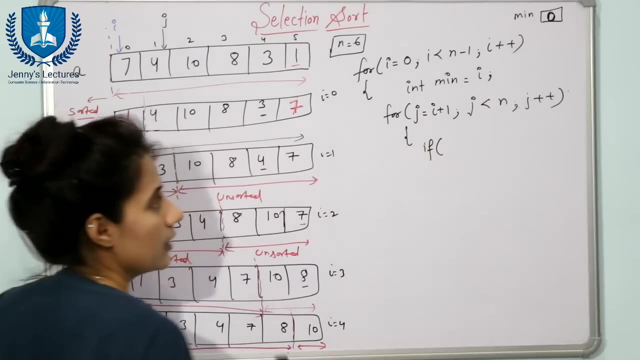 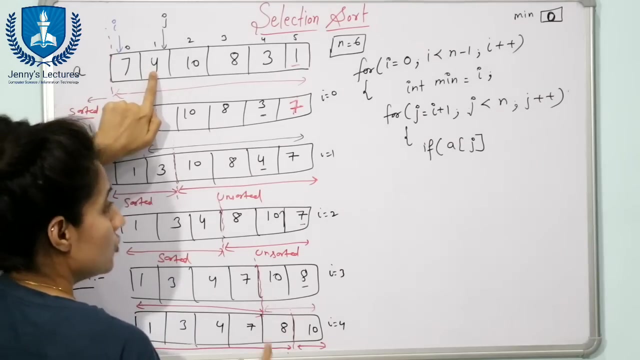 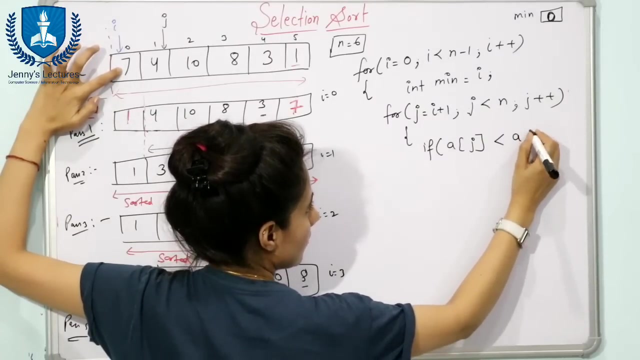 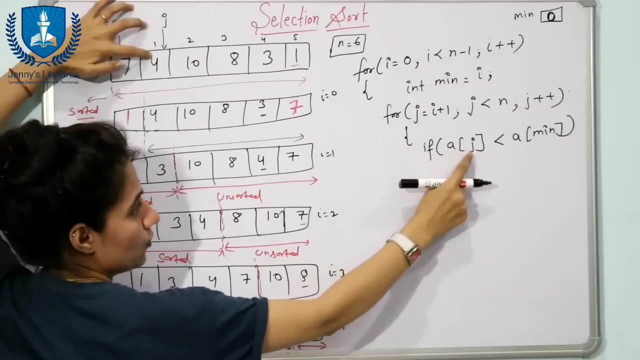 j would go what less than n? that is, till five. we are going to compare this seven with all the elements. so till n and j plus plus now. what to do? now? compare if, if this element, a of a of j, is less than this element. so now compare if this a of j, this a of j element, this element is less than a of min. see, min is what. 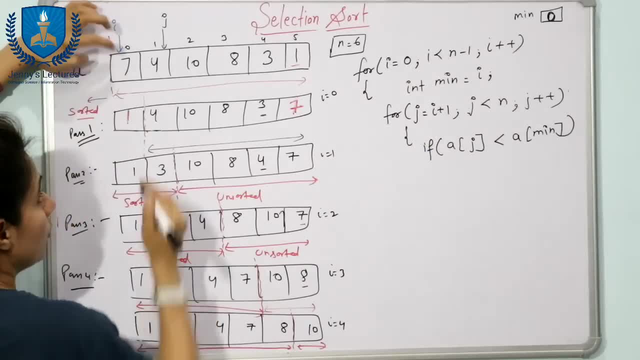 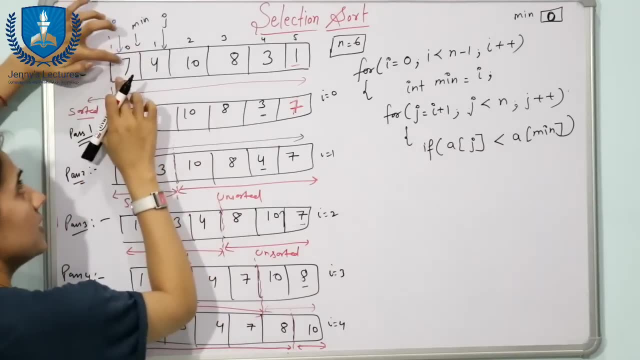 that value is i. so min is what here? only now min is at this place, only here only. okay, if this condition is true, if this element is less than this element, then obviously minimum element would be this one right at starting. we have considered this and this has minimum element. 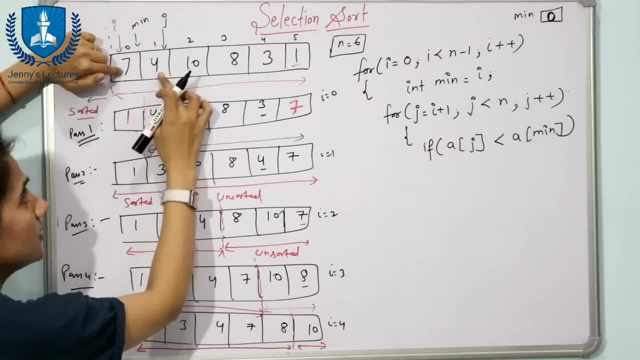 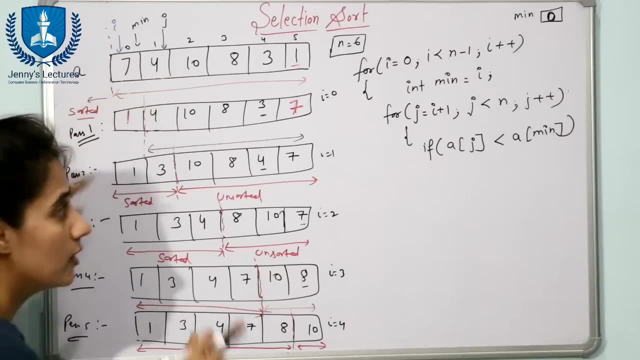 but if this element you find is less than this element that we have considered as in starting as minimum element, so minimum element would be updated now. so this is now the minimum element. so what you will do, you will do what minimum. you will update this min variable and min is equal to. 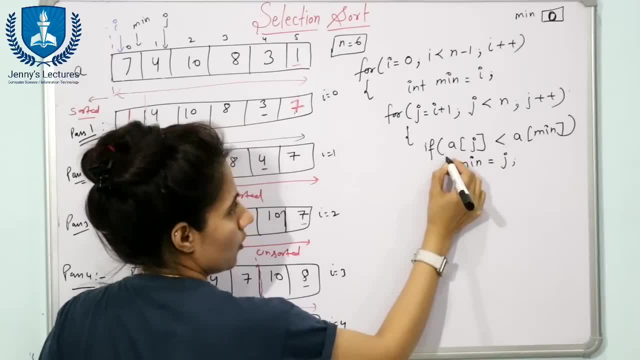 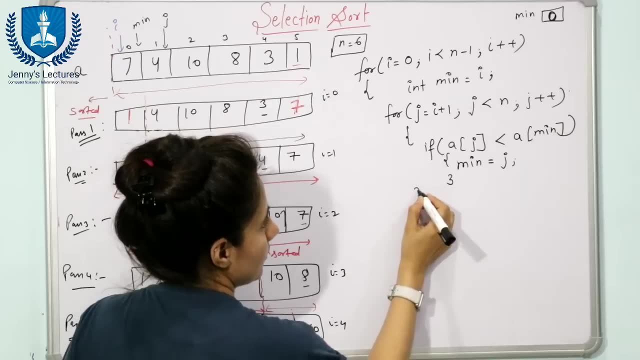 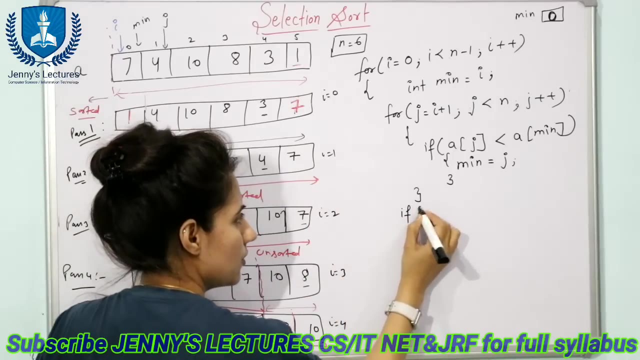 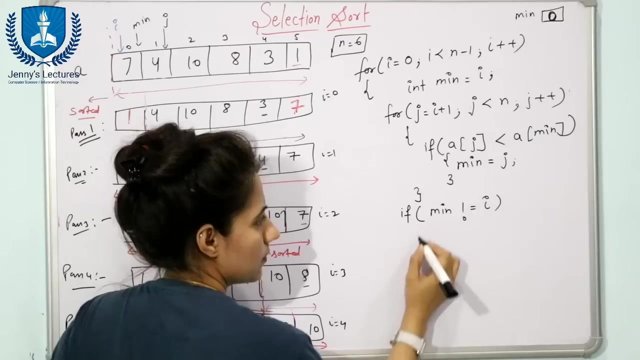 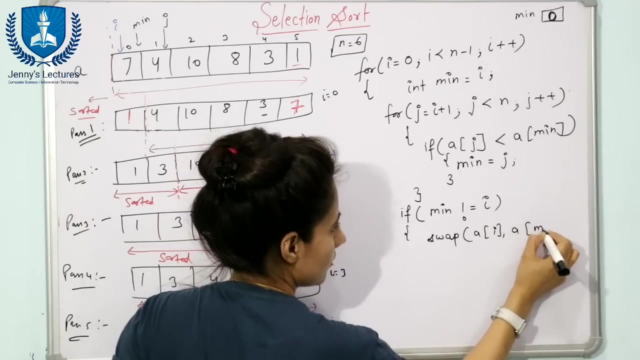 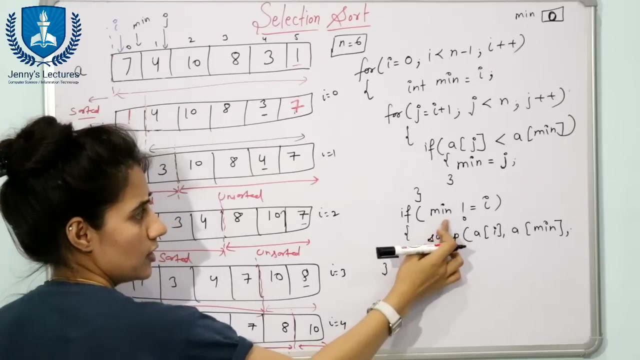 j now in, if you have. we have only one statement. okay, now see. now i will close this form loop and after this for loop, you will check if. if min is not equal to i, then what you will do: swap a of i and a of min. see why you are checking this condition. in starting, we have considered this. 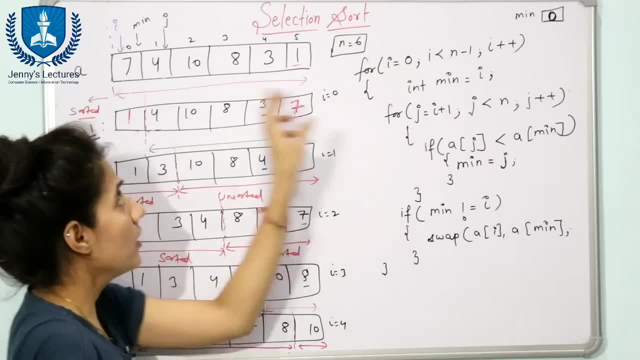 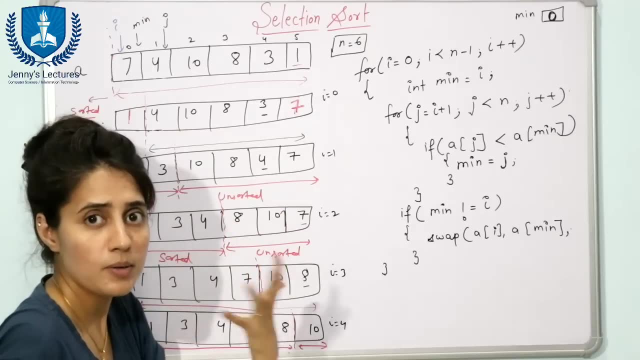 value. value of this main variable is same as i and j. so this is the value of this main variable and this is the value of this main variable. but when you are comparing this element with another elements, then you find out that some another element is minimum element. some another element is minimum than this element that we have. 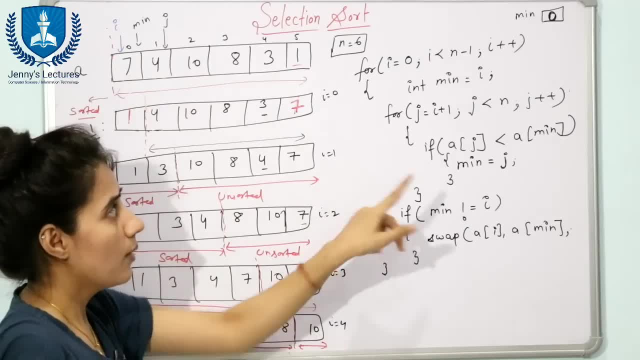 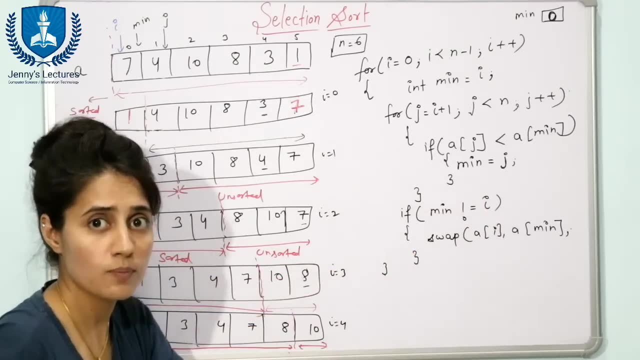 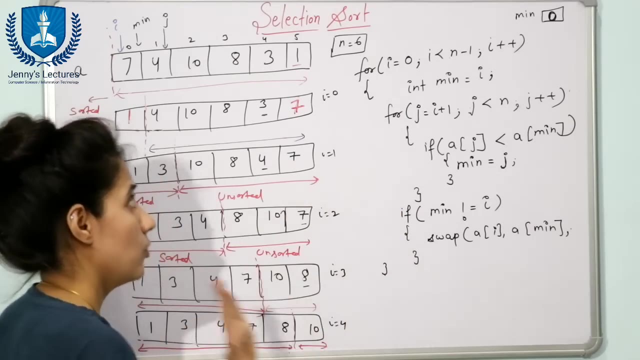 considered a minimum in starting. okay, so that is why we have- we have updated this min value, so min value and i value is not same. now, if min value and i value is not same, then you have to do swapping. in this case, we have done one swapping of one and seven. so see, let us trace out this code. 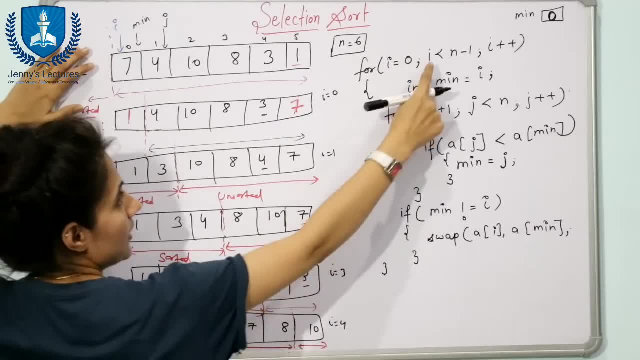 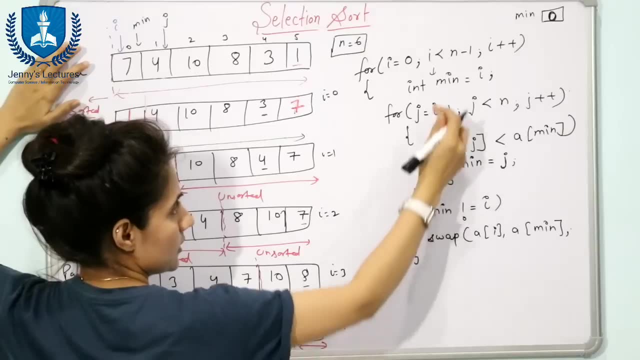 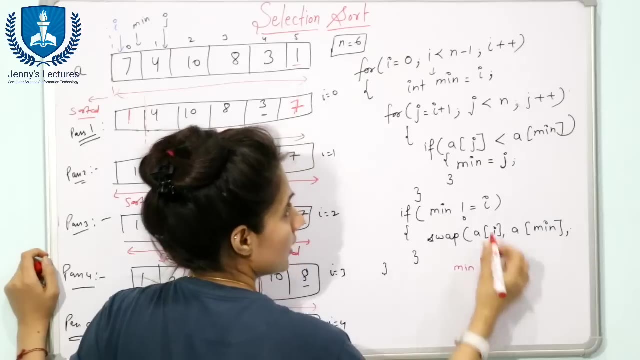 at starting. i value is zero. fine, i is less than equal to n minus one. yes, this condition is true. n minus one is five. zero is less than five. then we will go to this case into this for loop. so now see, min is a variable min and the value of this min is same as i. i is equal to zero. say min is. 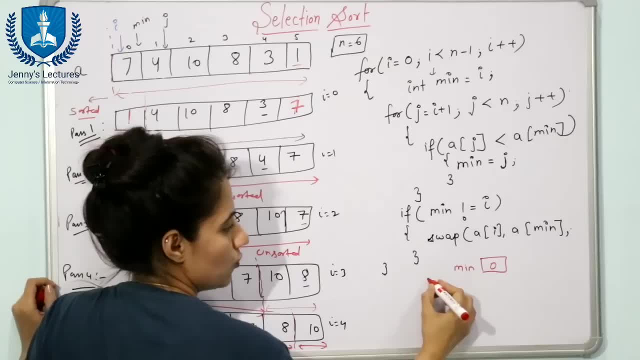 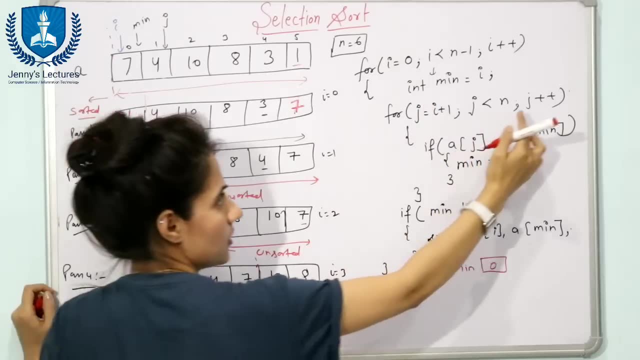 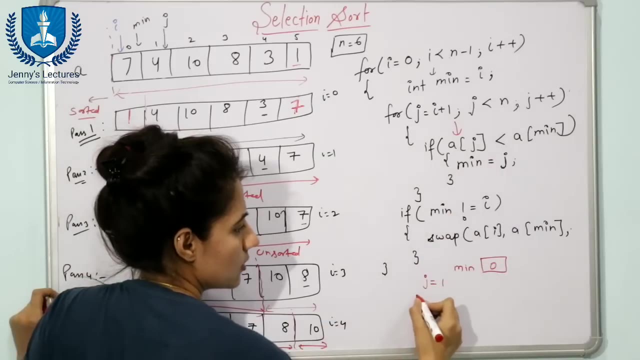 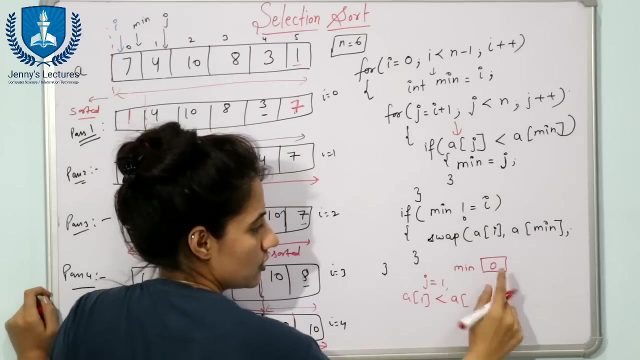 zero. now j is equal to i plus one. now j would be zero plus one. that is one and one is less than n, one is less than six, then that this condition is true, we will go, will go to into this loop now check if a of j, it means we are going to check a of one less than a of min min value is zero, a of. 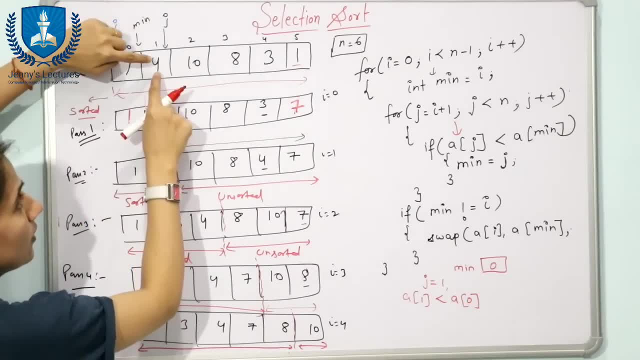 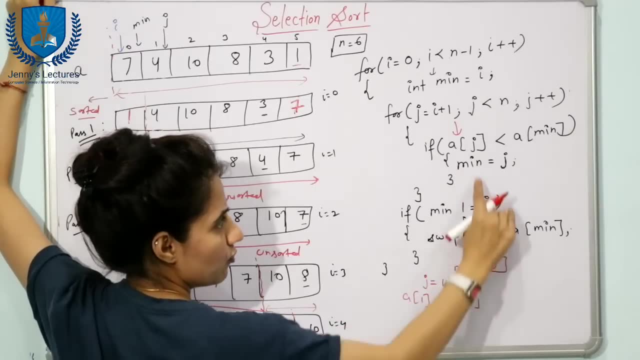 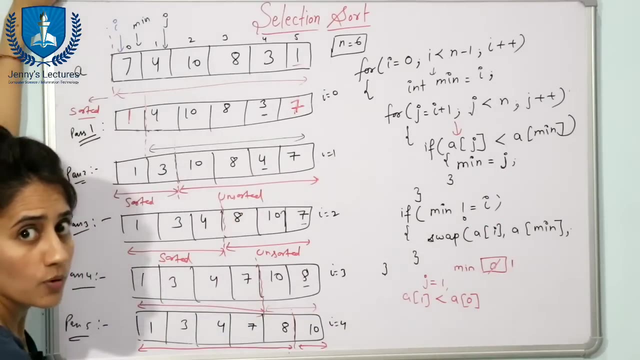 zero. now check a of one. is this one? this is less than this. yes, this condition is true. that is why we are updating this value of min now. min value of this min variable is j. now j value is zero, so this would be updated to one. now min value is one. okay, now see after this one again: j plus plus. 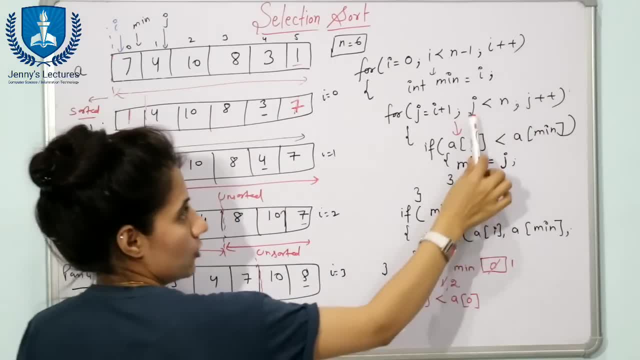 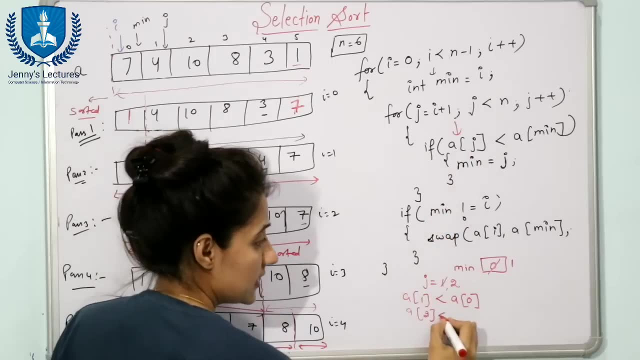 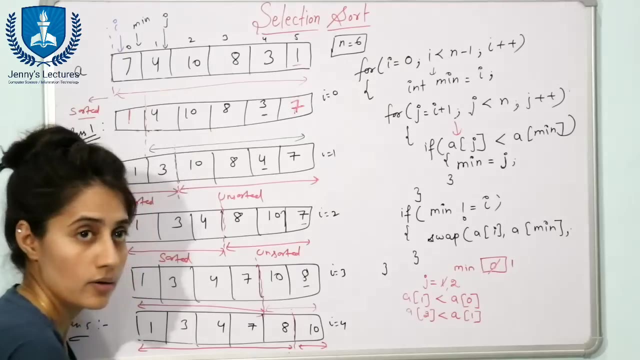 would be there. now j value is two. two is less than six. yes, this condition is true. we will go to this loop. now check a of two, a of j, less than a of min. now, min value is one. now a of one. see now a of two. 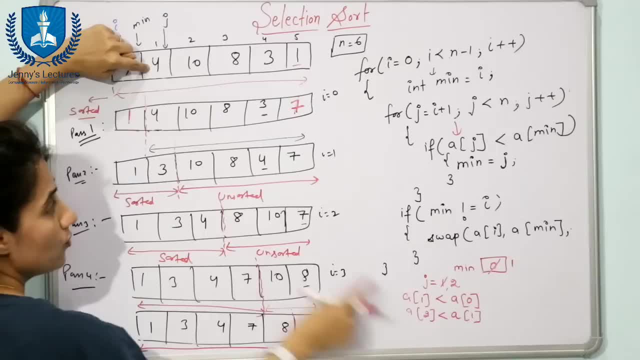 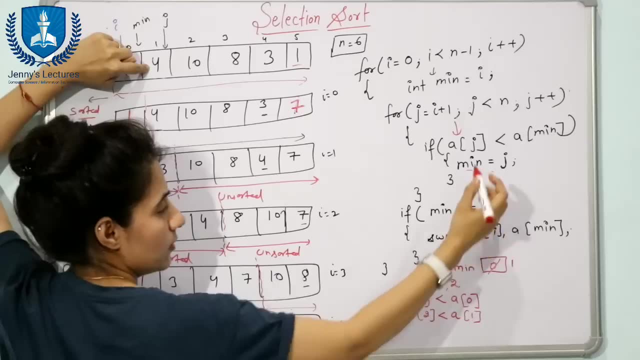 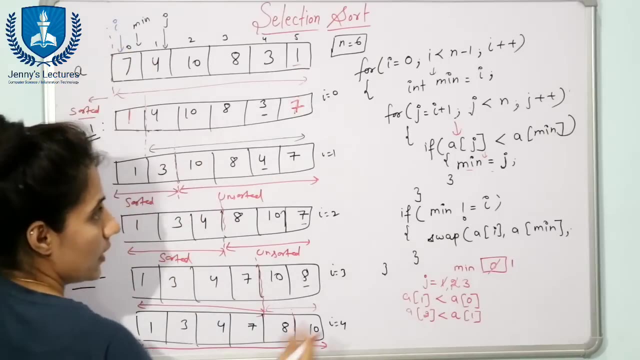 is a of two less than a of one. a of one is four. is this ten less than four? no, this condition is not true. so now min is not updated, because if this condition is not true, the control will not go within these statements. now again, j plus plus j is now three. now check a of. 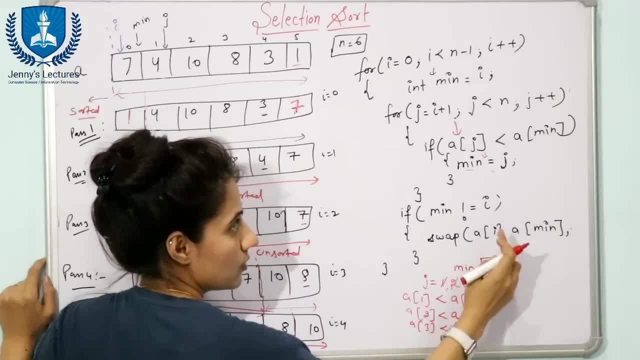 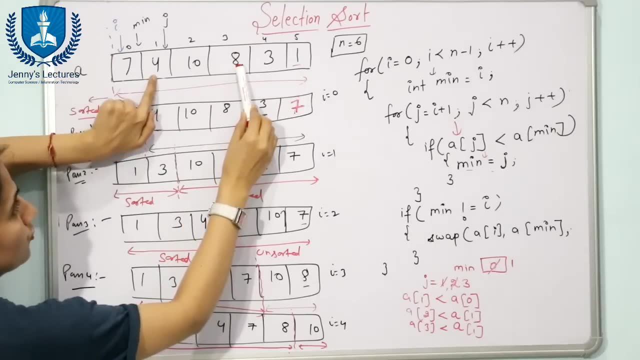 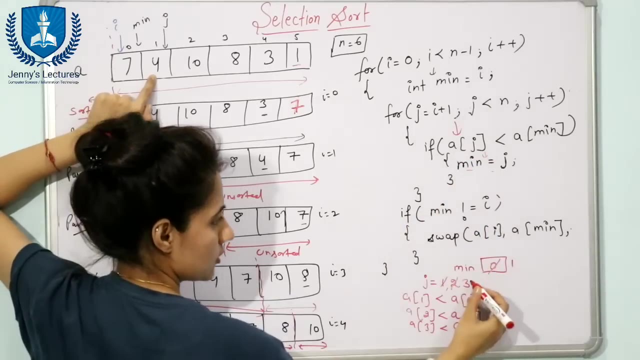 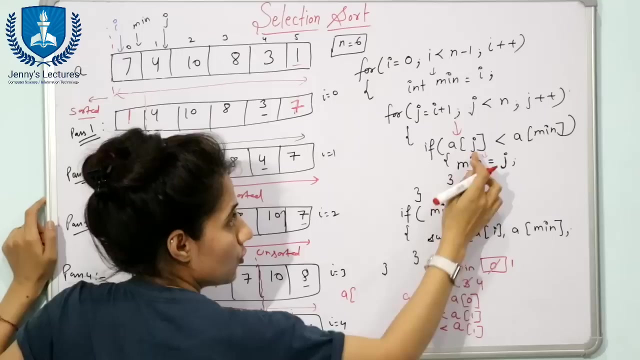 three less than a of min min value is still one. now check a of three. value is eight, a of one is: is this eight less than four? no, so we will not enter into this loop now. min will not be updated now. j plus plus j is now four. okay, now check a of four less than a of min value is still one. 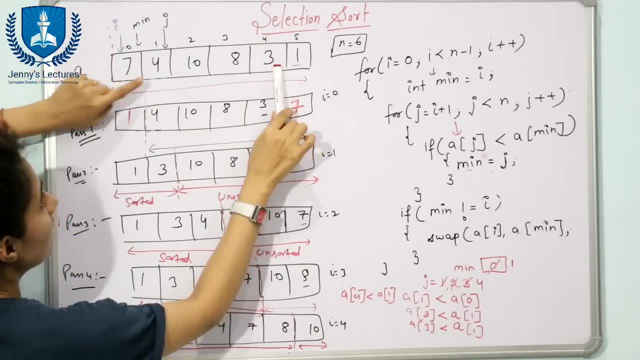 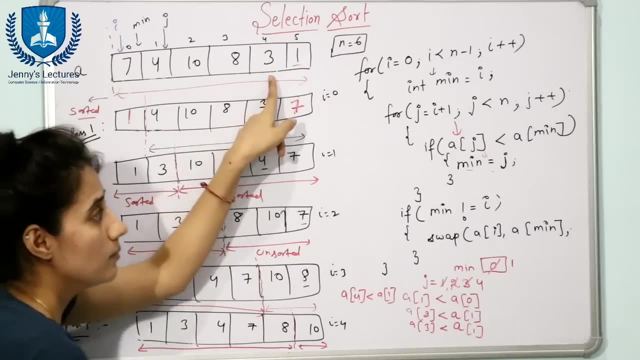 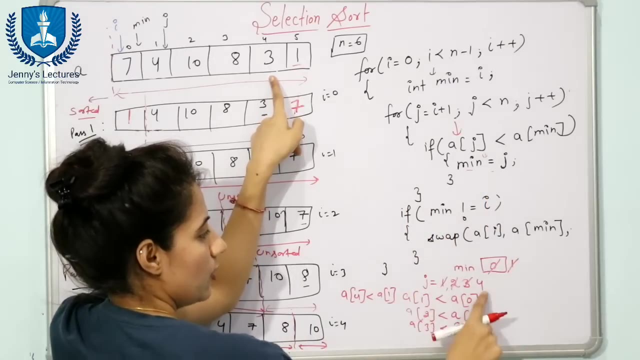 a of four is three and a of one is four. three less than four. yes, this condition is true. now minimum value would be: now we will enter into this loop: now j plus plus j is now four. okay, now check this loop into this loop. and now min is equal to j. now min value would be updated and j value is. 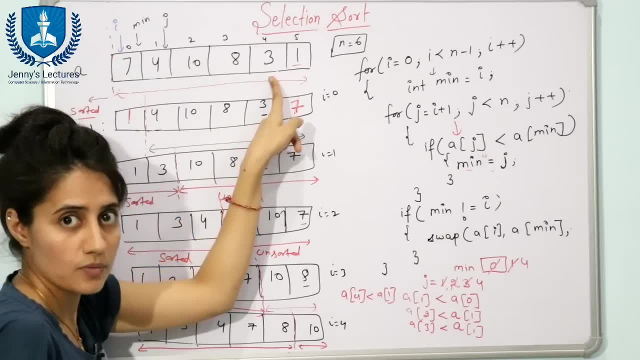 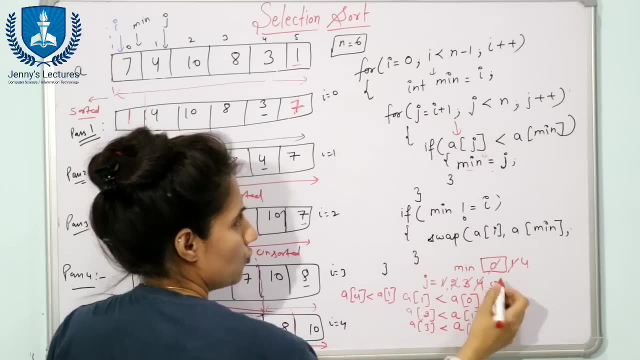 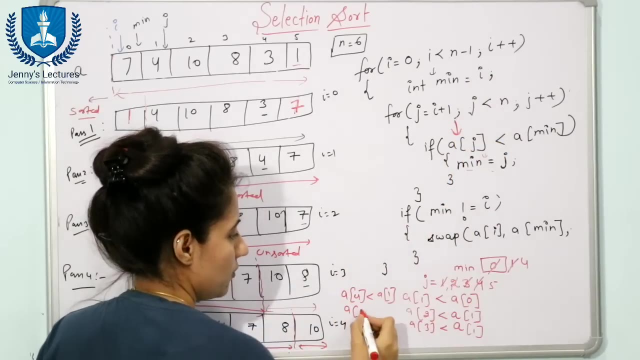 lot four. now mean value is four. okay, now, here we have that pointer, min pointer. okay, now see again: j plus plus j is equal to five. five is less than six. yes, condition is true. control will go to this loop. now check a of j. j is five, a of five less. 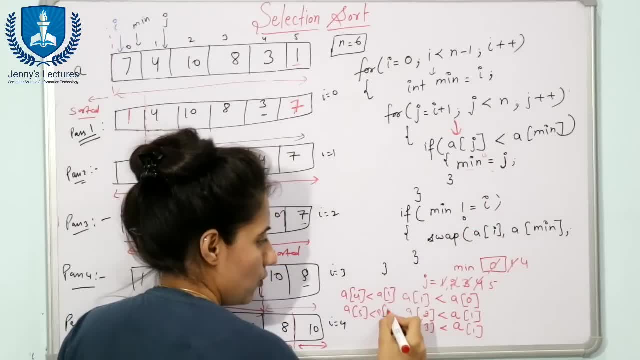 than a of min. now, min value is four. a of four, a of one is five: j minus j minus j plus squared j minus j. squared j of three is everything. meeting is no t two. just to to the blue click ah, p, orange, brown or t. circle is finished from t and y. 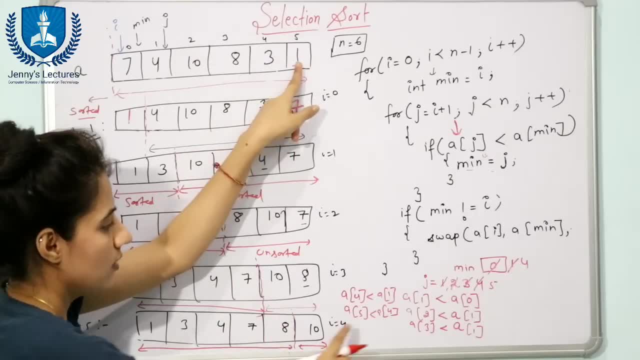 i object. dong c, dot, h, b. okay now, a of two was the interrupting per c that. delete that after�. rê of a of 5 is 1. a of 4 is 3. is 1 less than 3. yes, this condition is true. now control will go to. 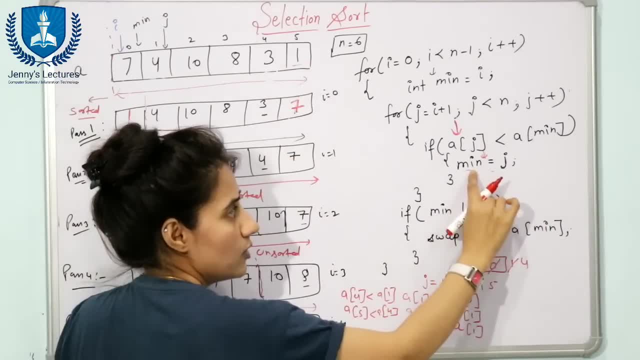 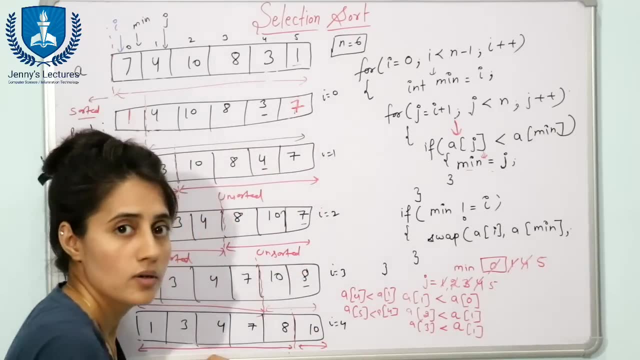 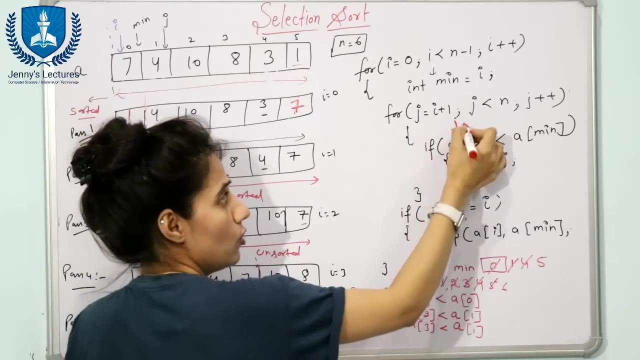 this loop. so obviously minimum element is this one, so minimum. the value of this minimum variable would be updated. and min is equal to j. now j value is 5, so minimum is equal to now 5. now again, j plus j is equal to 6. 6 is less than 6. no, this condition is not true. the control will not go. 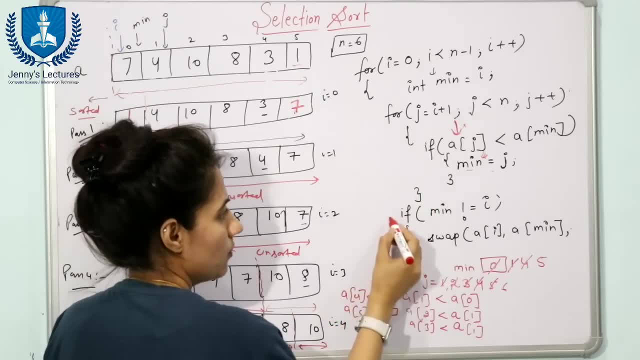 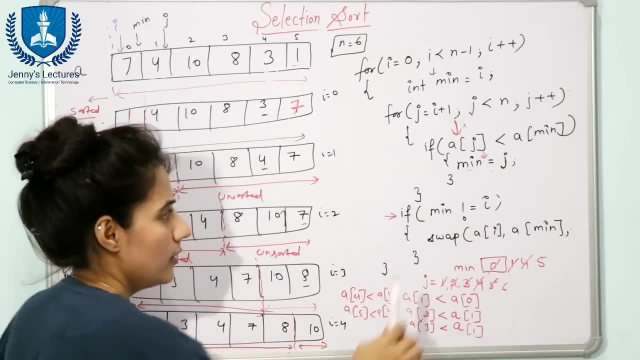 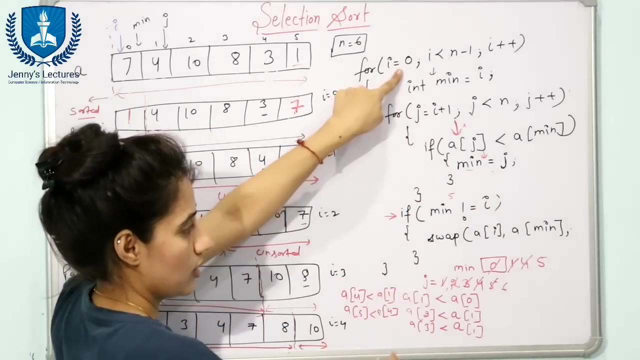 within this loop, control will go out from this loop and from out from this loop, the control will go here. only this is the statement. okay, now check if min not equal to i. now min value is 5, 5 and i value is. see, i value is 0 still. okay, we have started from 0. only i value is 0, so 5 is not. 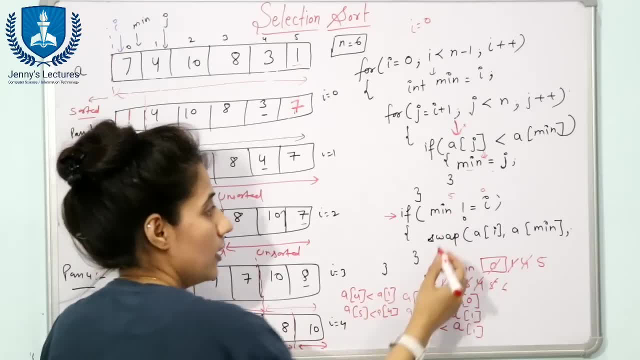 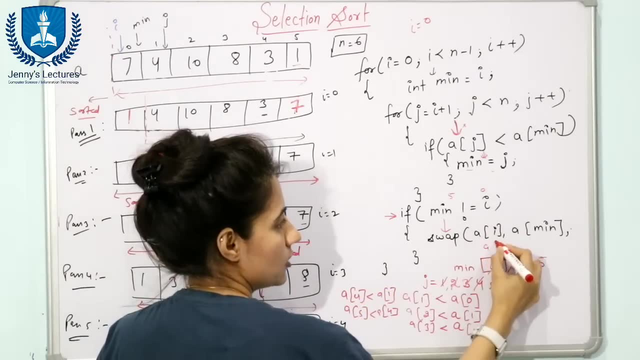 equal to 0. yes, this condition is true. fine, now we will enter into this loop. and what will happen? swapping of a of i, a of i. i means 0, means a of 0 and a of min is what 5 value of min is 5. 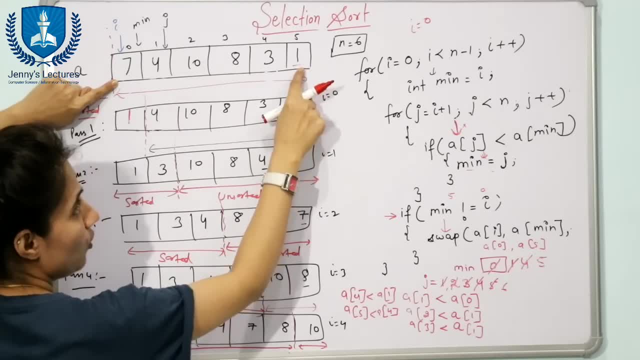 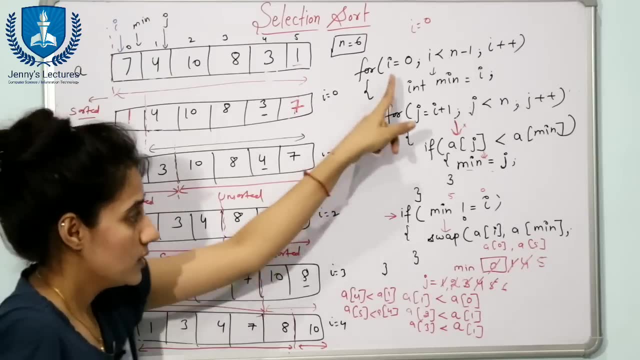 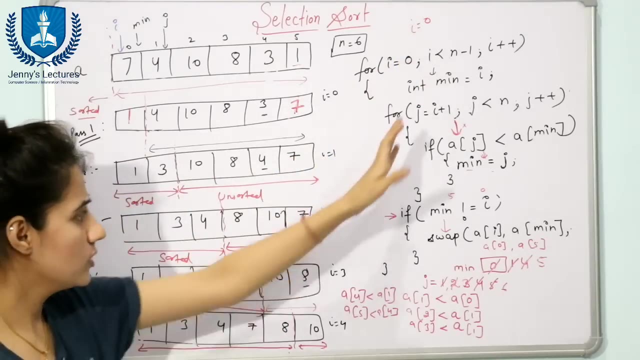 so now a of 0 and a of 5 swapping of this one, 1 would go here, 7 would go here and that's what we have done. okay, so this is the code for this selection sort. so you just take out another case also i value you can take 1 or 2 and you just trace out this code and find out that this. 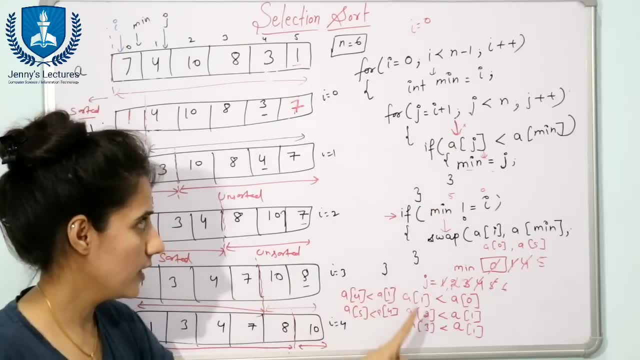 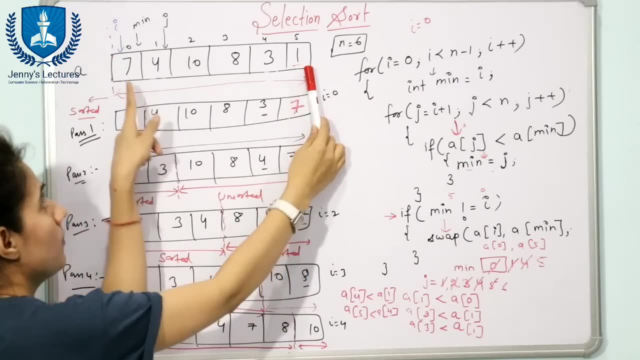 code is acceptable, absolutely right. i have just taken one case and i trace out this code with that case and we have find out that we have after this: after executing of this code, one would be swapped, one would be swapped with 7, and that's what we have done. when we are discussing this numerical without 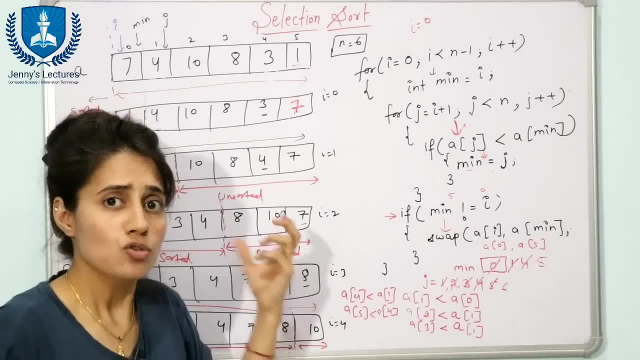 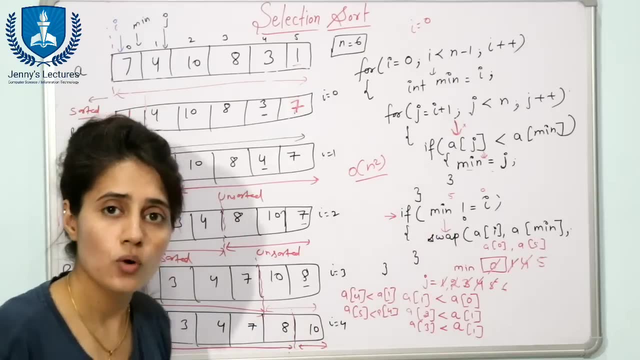 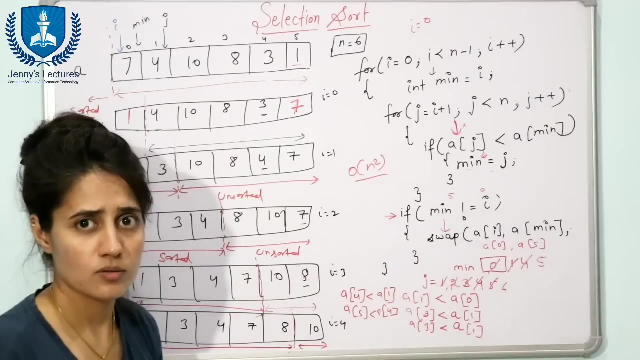 this code. so what about the time complexity? so the time complexity of selection sort is order of n square, both in worst case and best case, because of the time complexity of selection sort is order of n square, can see how many times this inner loop would be computed. obviously n square time. fine, because